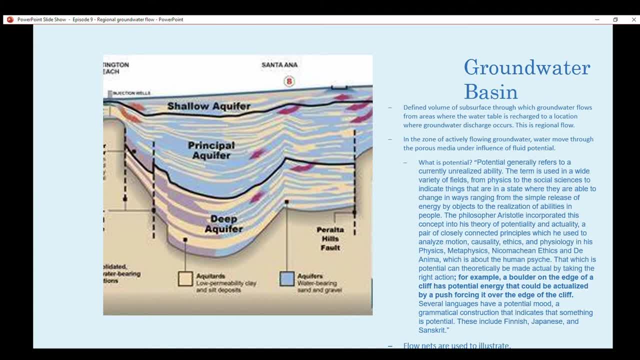 front to a location where the groundwater discharges. So a stream in a basin- a sedimentary basin is the best way to think about it- like a basin in range, Prototypical, normal faults on both sides, with maybe a stream in the middle And this is called regional flow. So in the zone of actively. 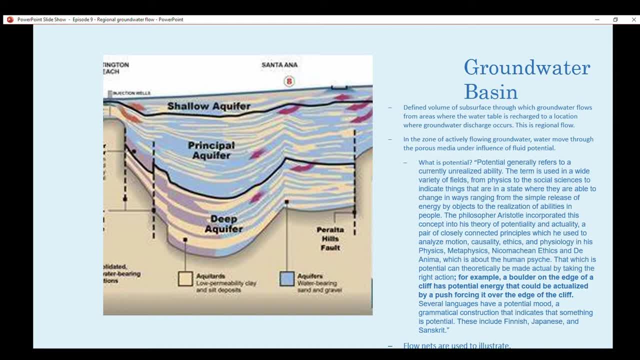 flowing groundwater. the water moves through the porous media under the influence of fluid potential- and I'm not going to read this whole thing, It's a throwback to physics. But basically the potential is what refers to an unrealized ability, And I bolded this part because it's a good example. 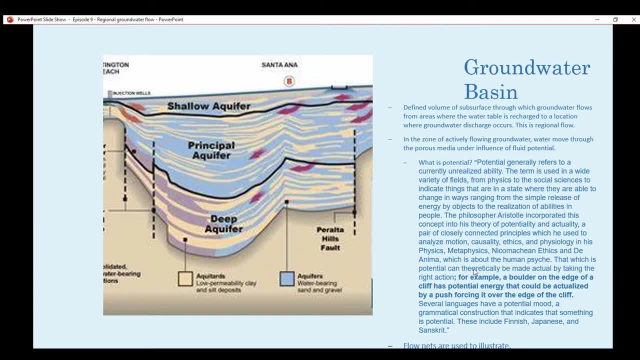 So a boulder on the edge of a cliff has potential energy that could be actualized by pushing it off the cliff, And at that point it's not potential energy anymore, it's mechanical energy. But anyways, flow nets are used to describe regional flows and, in terms of recharge, 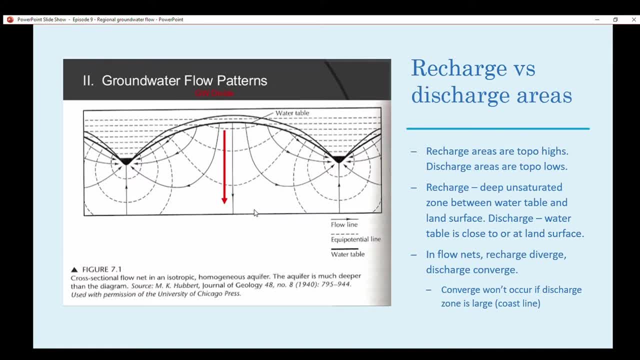 versus discharge areas. you have well, recharge areas are typically topo highs, so topographic highs- mountaintops, hills- and then discharge areas are topo lows such as valleys- yeah, valleys, that's the best way to think about it. a recharge, so recharge, talking about the deep unsaturated zone between the water table. 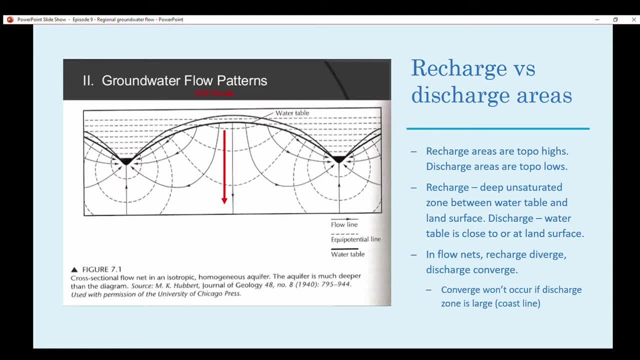 and the land surface and okay, sorry I'm reading that wrong. so in deep unsaturated zone between the water table and the land surface. that's significant for recharge, whereas discharge is a deep unsaturated zone between the water table. the water table is close to the land surface, so you'll have more discharge. 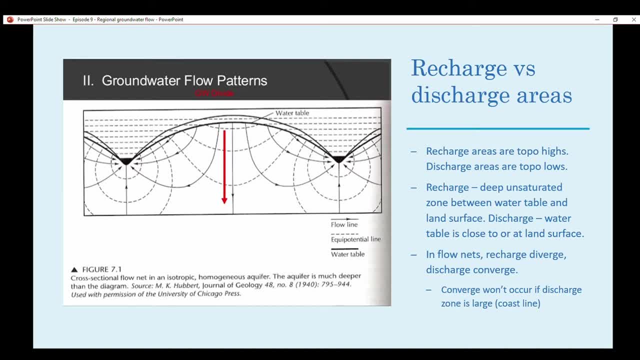 occurring due to evaporation or it's closer to the surface. so if you have a change in topography, that you can have a spring form. if flow nets- and well in flow nets- recharge such as okay, this is moving, slow recharge, they diverge. so basically, think of it like this: at the top, that's a that's diverging, and then 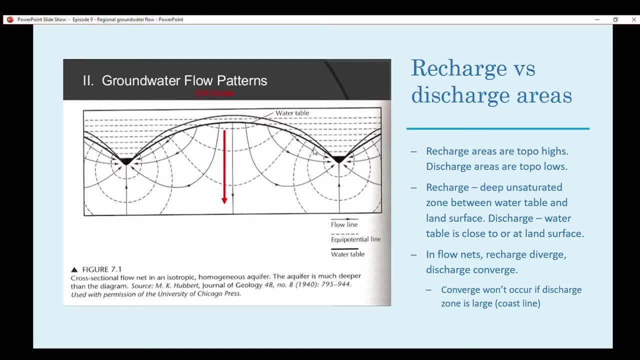 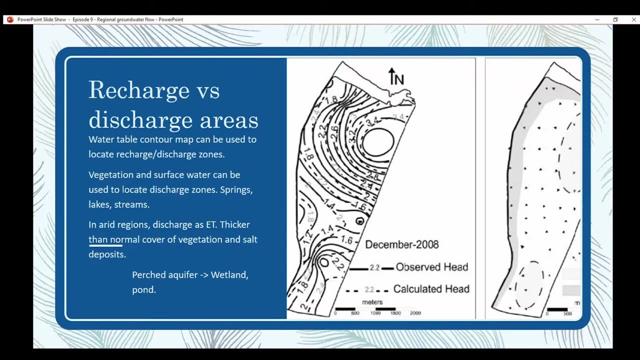 discharge into the stream valley is converging. those arrows, those flow net arrows. converge won't occur if the discharge zone is large, such as at a coastline. so recharge, whoops. so recharge versus discharge areas. the water table contour map can be used to locate recharge and discharge zones, vegetation. 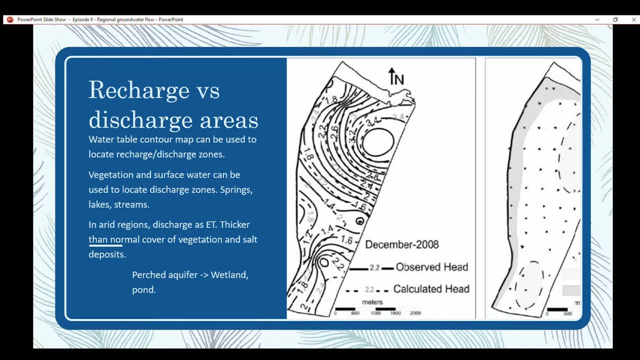 and surface water can be used to discharge zones, and that's because, obviously, vegetation is going to grow where there's water and in an arid region, as you'll see on the next slide, I'll show you what that means. but you, springs, lakes and streams are discharge. 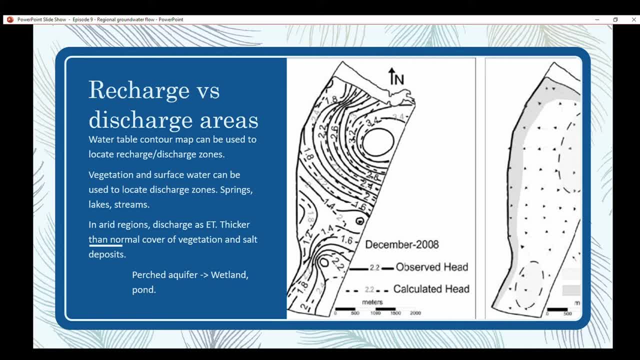 zones. so when we're talking about surface water, we're talking about springs, lakes and streams. so in arid regions discharge occurs as evapotranspiration. it's thicker than normal cover of vegetation and you might have salt deposits occur at a discharge zone and a perched aquifer could lead to a. 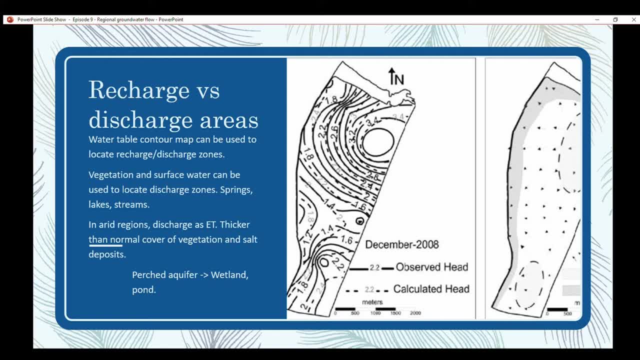 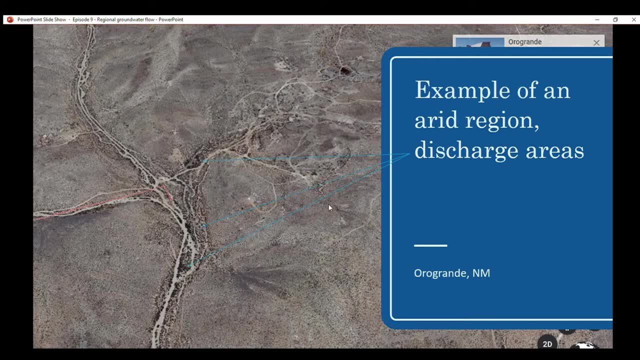 wetland or pond, and so this is one of my favorite places in in this region of the country. so Oro Grande is a very, very dry place typically, but it has some beautiful streams. it's known for its former mining district, but it has some beautiful streams that cross-cut it. 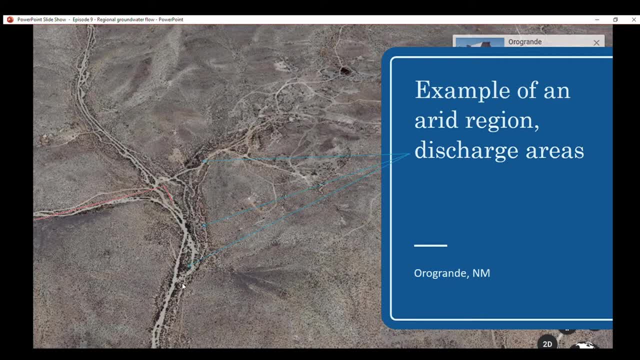 and I mean you can see the vegetation density occurs along where the streams are. that's where the water table is most likely the highest. so obviously it makes sense that vegetation is going to be at its thickest density along these stream areas. so in humid regions the water table follows the topography. 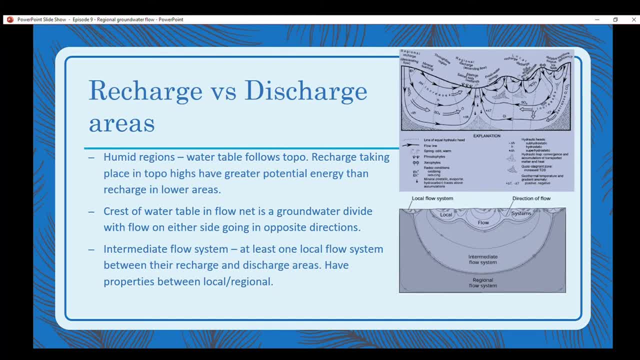 for the most part, recharge takes place in topographic highs and it has greater potential energy than recharge in the lower areas. crest of the water table and a flow net is a groundwater divide with flow on either side going in opposite directions. I did not picture that here. I think it's on the next slide, but an 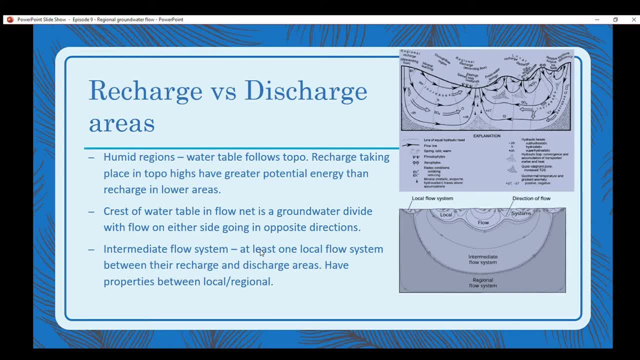 intermediate and we'll go through the ok. so there's three types. there's regional flow systems, intermediate and then local. so an intermediate flow system is it's at least one local flow system between their recharge and discharge areas and it has properties between local and regional. so it's basically obviously intermediate. it's between what a local flow? 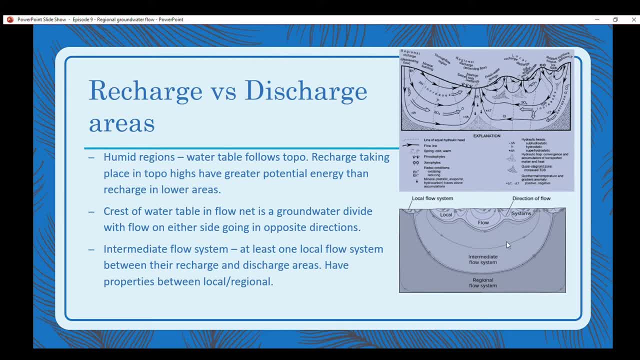 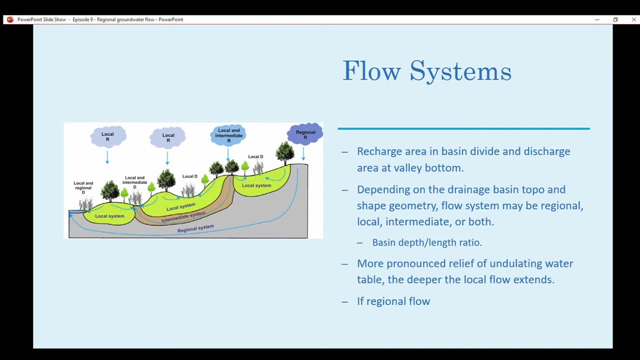 system is and what a regional flow system flow system is. so a flow system, so a flow system. and this is a good picture of a local flow system: recharge area in the basin divide and discharge area at the vet Valley bottom. that's talking about a regional. it occurs here. 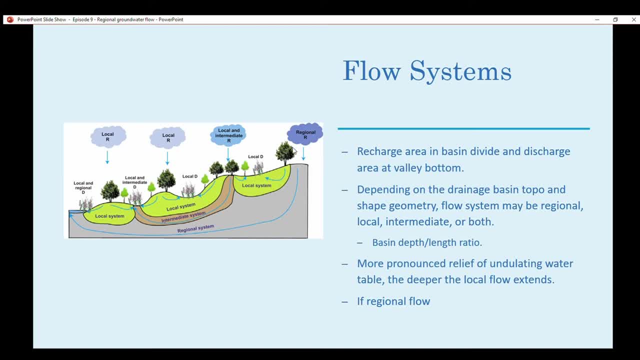 on the mountain front or hit the top of the hill and it slowly makes its its way to what is basically a lake or a river over here, and when you're talking about a local system, it's very small flow paths and close to the surface. okay, I'm getting ahead of myself. 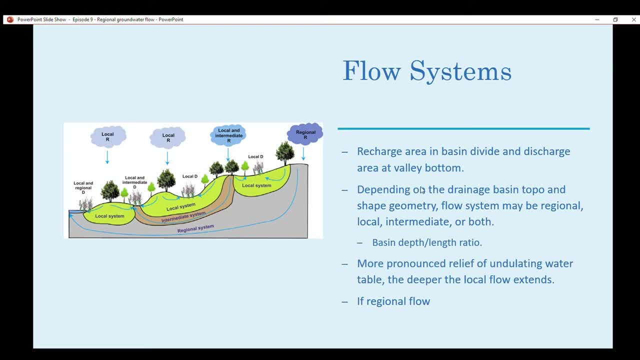 but uh, depending on the drainage basin, topography and shape, geometry for the flow system may be regional, local, intermediate or well, all three and it base in depth and length ratio can affect a which one you'll have more pronounced relief of undulating water table the deeper the local flow. 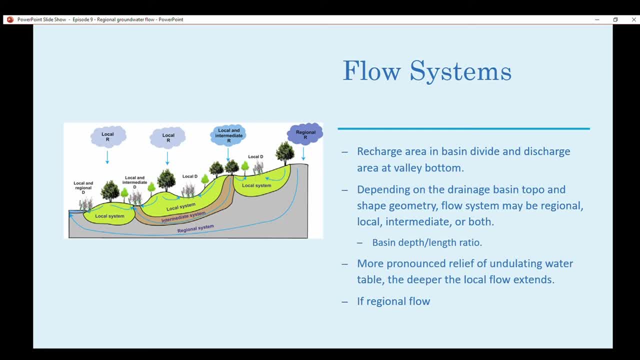 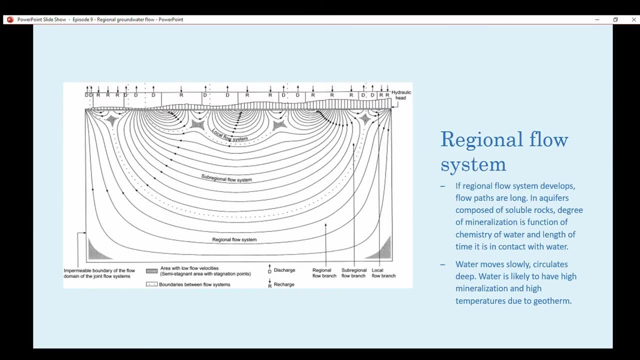 extends and I did not finish that sentence. okay, I'm just continuing it on the next one. okay, so the regional flow system. if the regional flow system develops flow paths uh are long as you can see, and these take thousands, millions of years to travel. uh, it's actually going uh right to left the uh the regional flow system. 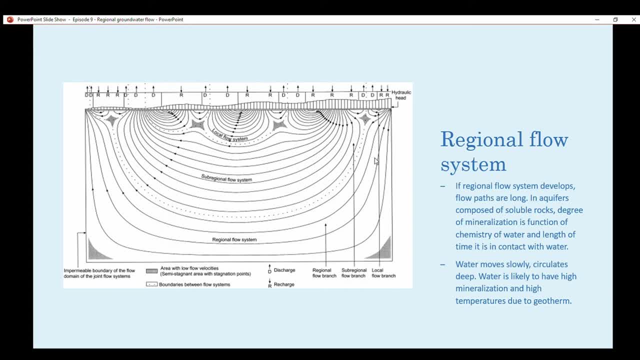 um, it travels really deep into the uh into the lithosphere and comes back up and uh in aquifers composed of soluble, soluble rocks such as limestone. the degree of mineralization is a function of chemistry of water and the length of time it is in contact with water. so if you have something flow uh, groundwater flowing through a regional flow. 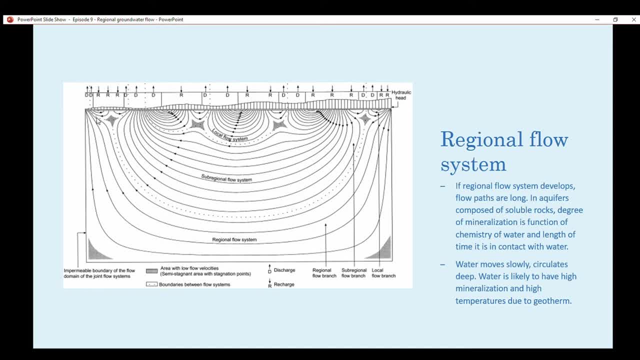 system and it's flowing through limestone. it's going to be really hard water, really, really really undrinkable water by the time it reaches the top, and that at that point it could be a travertine deposit or it could be uh, could be, uh, just a deposit of calcite. 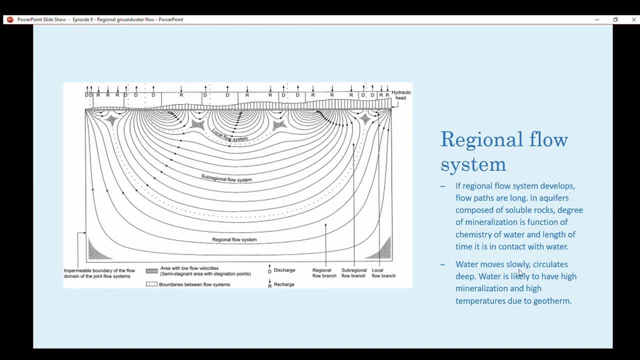 um. so water moves slowly and it circulates slowly and is likely to have a high mineralization and high temperatures due to the geotherm. obviously you go deeper into the crest the warmer it gets. but also as groundwater flows through rocks, that heats up due to friction and it's trying to overcome the friction, so it's heating. 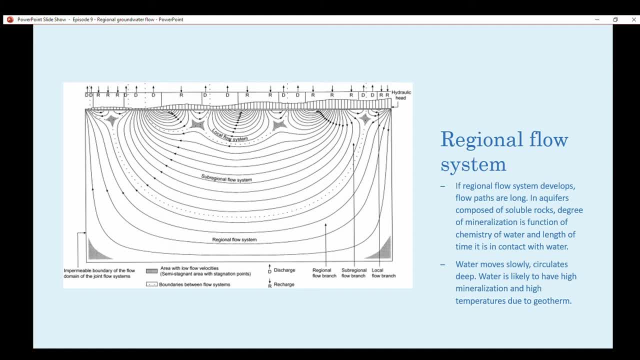 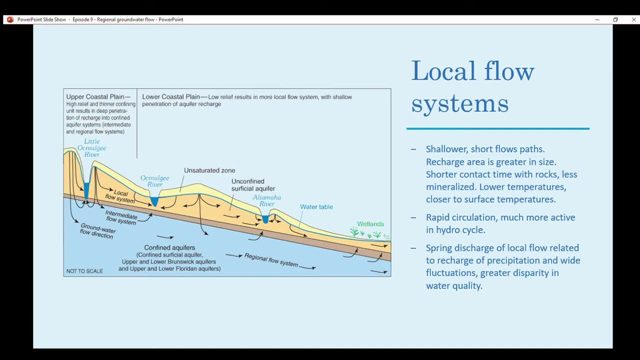 up that way too. and when we're talking about a local flow system, it's much shallower and it has short flowpaths, its recharge area in size, the shorter contact time with rocks and it's less mineralized. you have lower temperatures, which it's closer to surface temperatures. you have rapid circulation, so it's much more active. 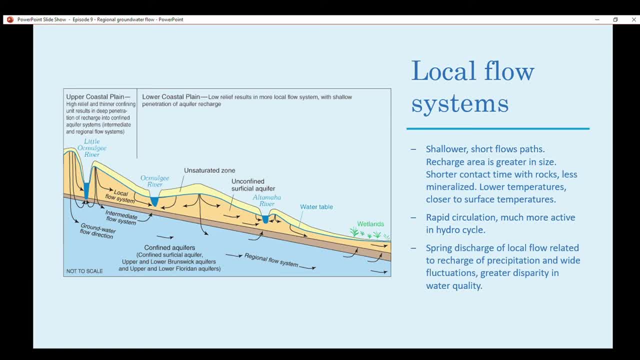 in the hydrologic cycle and spring discharge of local flow related to recharge of precipitation and wide fluctuation. wide fluctuations, which creates a greater disparity in water quality. and this is kind of a cool little cross-section showing three different rivers and because they're so close together, it's considered a local, local flow system. short paths and you. 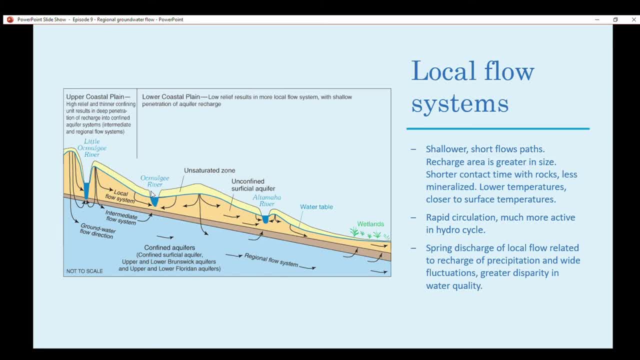 have you know, this was pretty interesting- and eventually reaches wetlands, in this particular case from the Altamaha River, so slowly makes its way to wetlands well quickly, quicker than a regional flow system which is shown built, but in this confined aquifer. this is a confining layer. so in terms of non-cyclical groundwater, you have fossil water, which is water. 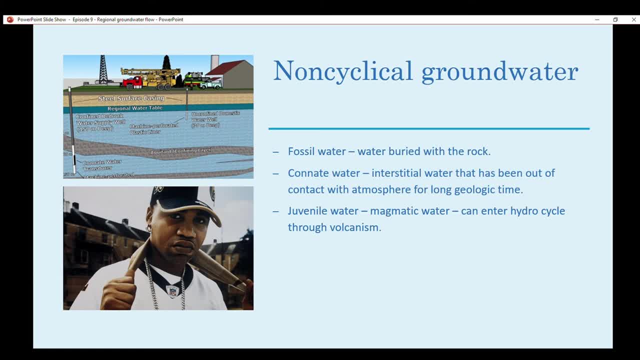 buried with, with the walk with the rock, you have conate water, which is something you hear about when you're dealing with petroleum geology. that's that's water that they typically come in contact with when they're drilling for for oil. it's interstitial water that has been out of contact with the atmosphere for